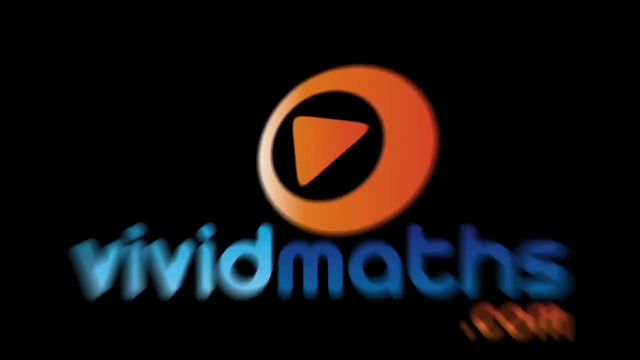 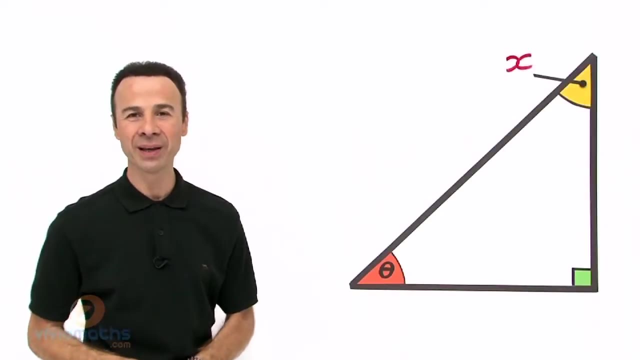 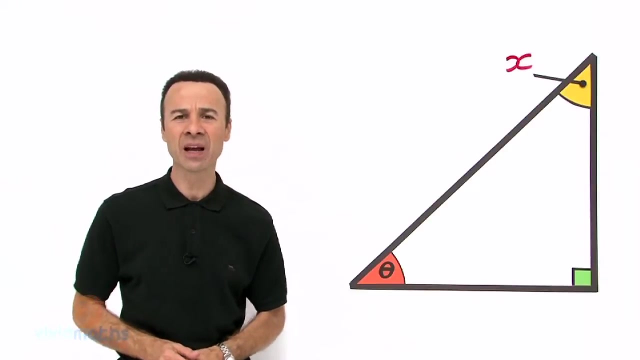 Hi guys, have you ever been in a test and they give you this question and you look at it and you are kind of confused and you are thinking: how do I do this? They haven't given me enough clues in the question. Like you look at the question and you say, well, this. 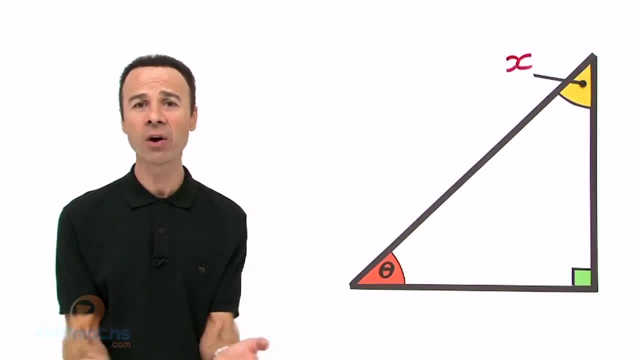 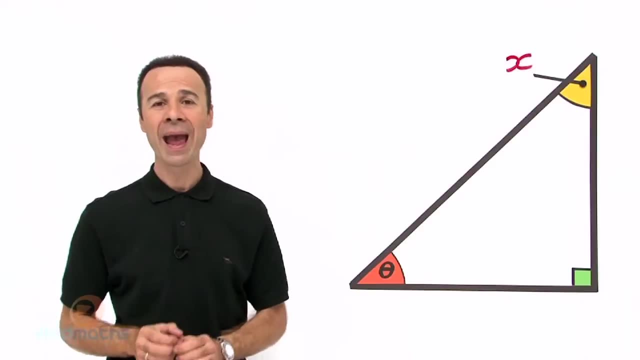 minimal, meager, limited information. how can I possibly work this out? Well, if you like to know how to do those guys those types of questions, I am going to show you in this example how we can exercise our resourcefulness, how to be more resilient and how to respond. 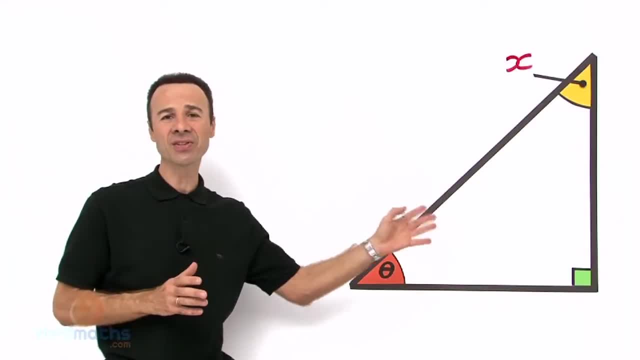 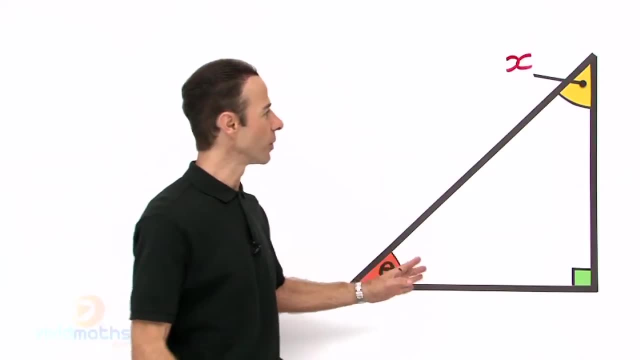 to these types of questions where the information is so limited. and this is a classic example: right here on my left, As you can see, we have a right angle triangle, so we have limited information. basically, they haven't given us any numbers, have they? and they say: well, 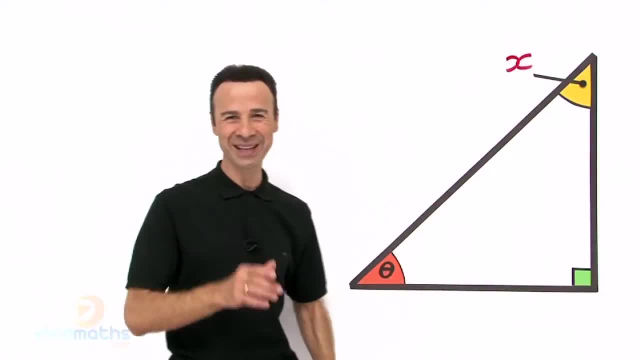 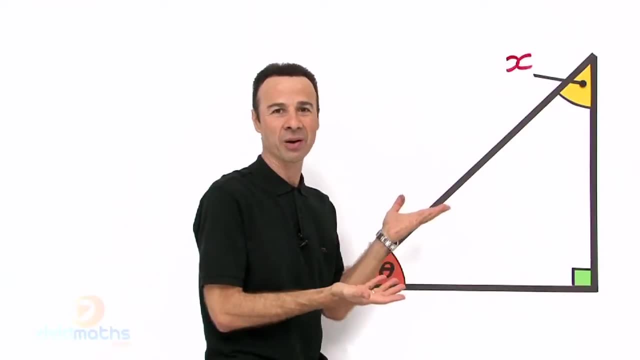 we want you to find out what x is up here and we are not going to give you much information. and you look around yourself, say: well, we just got theta here and we got a right angle and it is a triangle. well, what can we do? 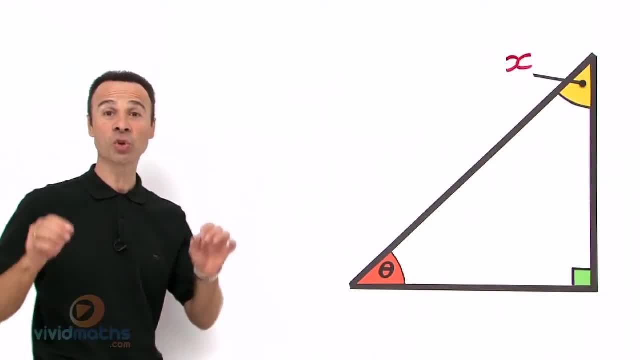 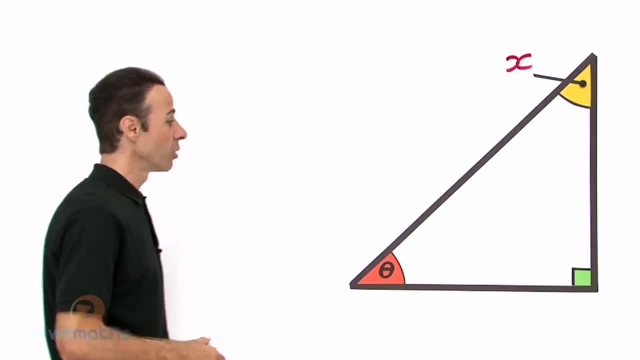 Well, let us be resourceful. first step in answering these types of questions is to write down what you do have. write that down. even if it seems meager and limited, write it down. So let us see what we do have. well, one of the things we do have is: well, we got a theta. 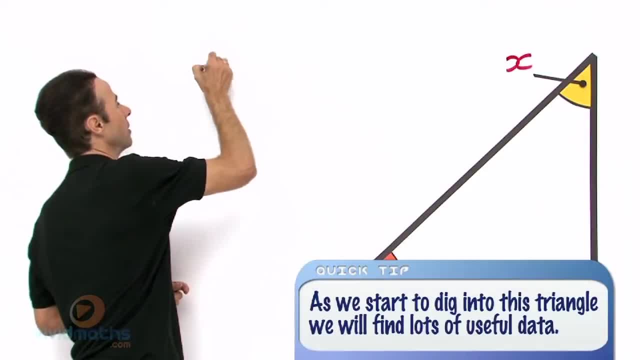 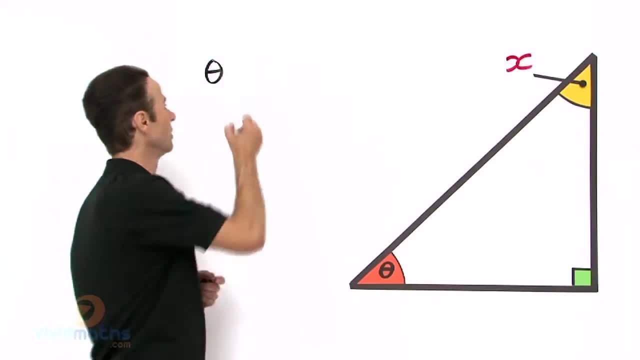 there. it does not sound like much, but let us write it down. we have theta. yes, let us celebrate. we have a theta. Now, what else do we have? We have 90 degrees. right there, it is a right angle, so let us write that down- plus 90 degrees. 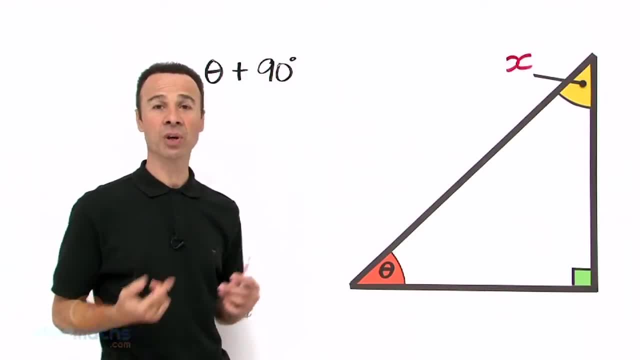 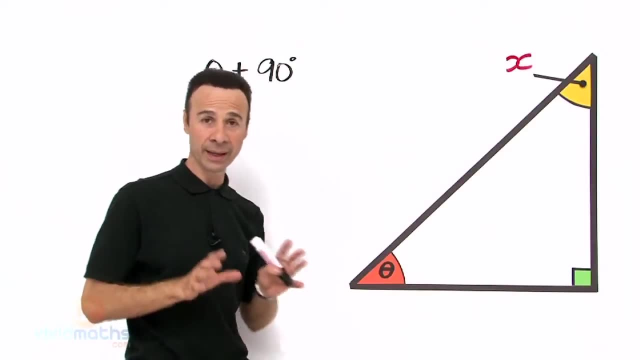 Okay, now do we know something about triangles that we could use here, for example, some sort of strategy. one strategy we can use is: we know that all the angles in a triangle add up to 180 degrees. yeah, So we could use that, couldn't we? 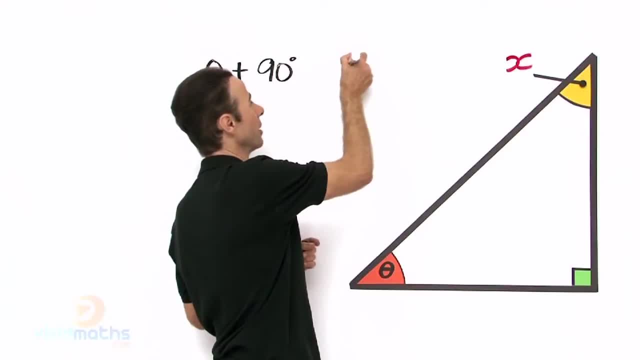 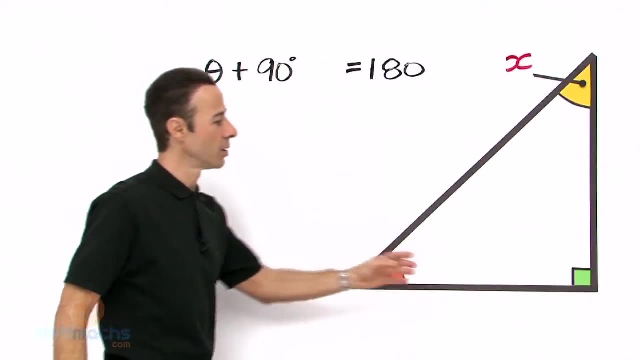 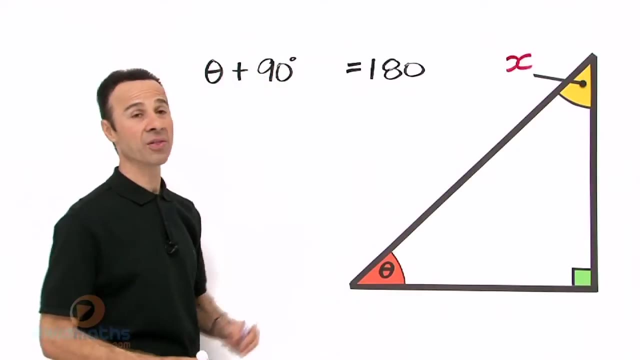 So all these angles, let us write that down. If all these angles… If all these angles equal 180 degrees, that means theta right here, 90 degrees right angle right here, plus the missing pronumeral X right over here. we could just add those three. 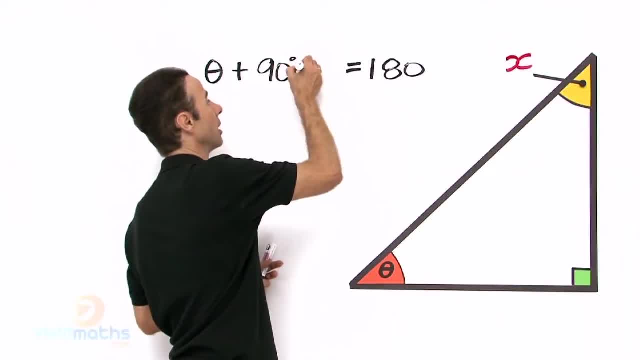 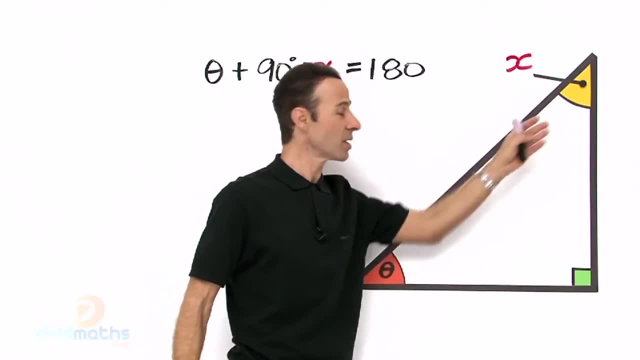 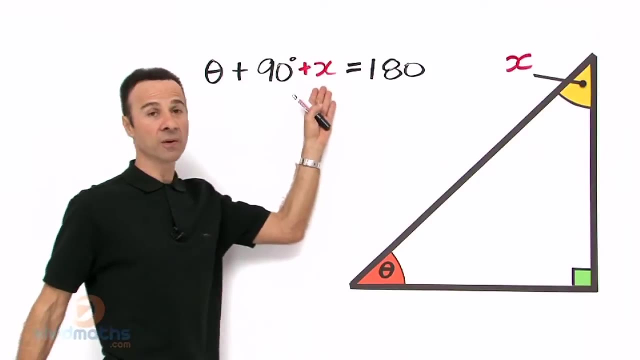 together and it will equal 180 degrees. let us do that plus X. Okay, theta plus 90 plus X 180, theta plus 90 plus X 180. that seems very plausible and very practical. Now let us get X. Let us get that by itself, because that is what we are asked to do, we are looking for. 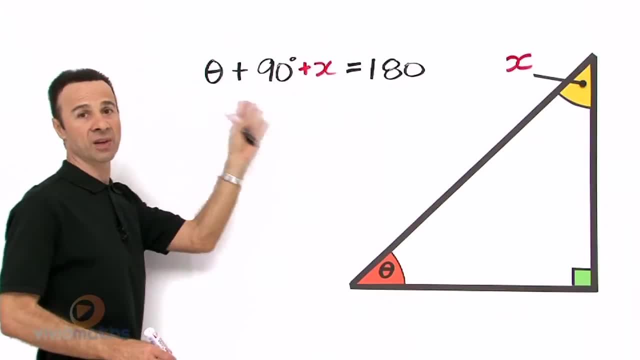 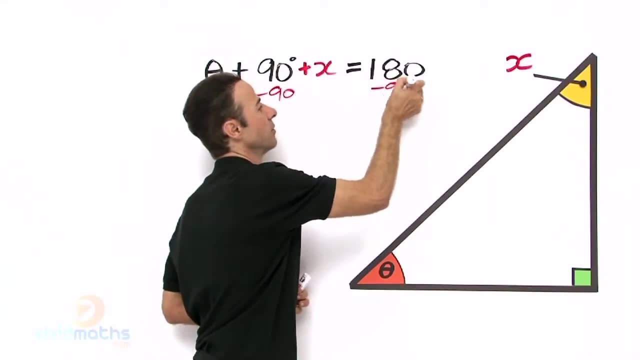 this missing pronumeral. Let us get that by itself. let us get rid of these guys over here. yeah, So how about we take away 90 from both sides? So we take away 90 from here, take away 90 from there, which leaves us just with a theta. 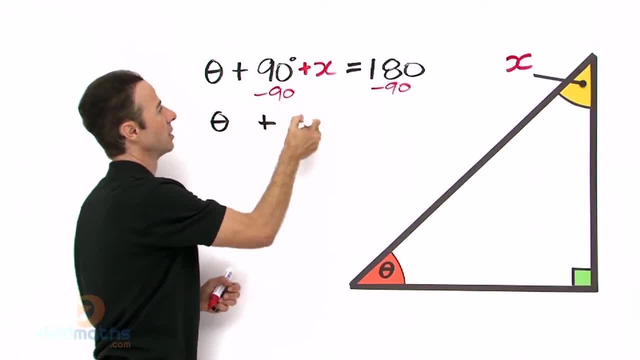 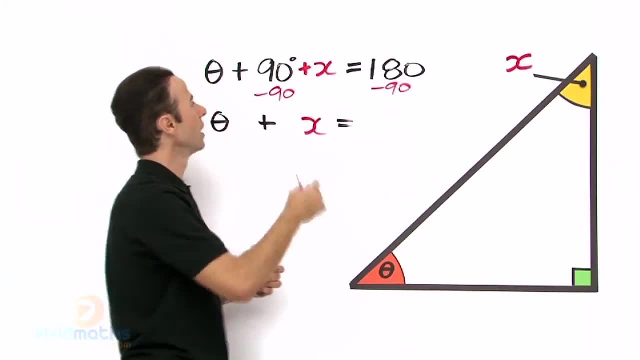 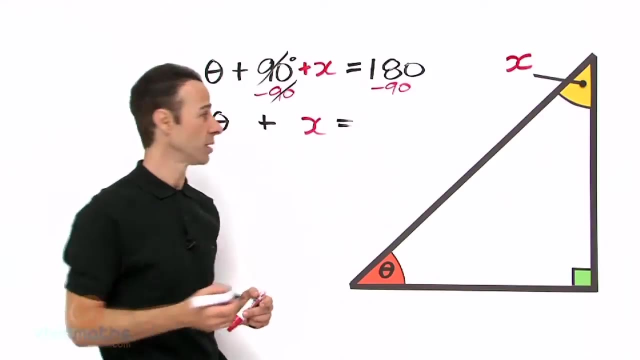 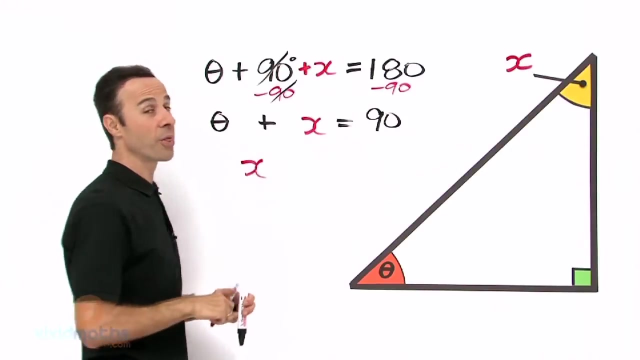 over here, theta plus X from up here, and that is going to equal well, 90, 90, cancel, cancel, cancel. So 180 take away 90 leaves us with a grand total of 90, okay, Now let us bring the X over here and take away theta from both sides. so take away theta. 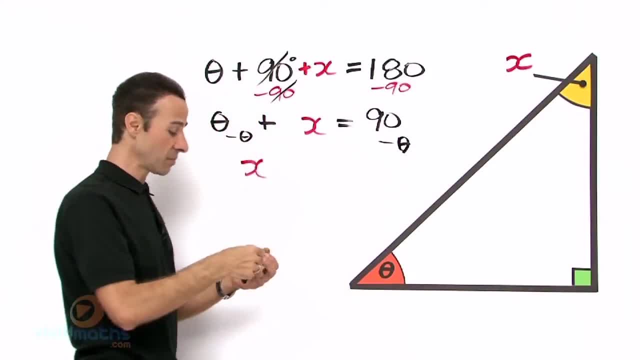 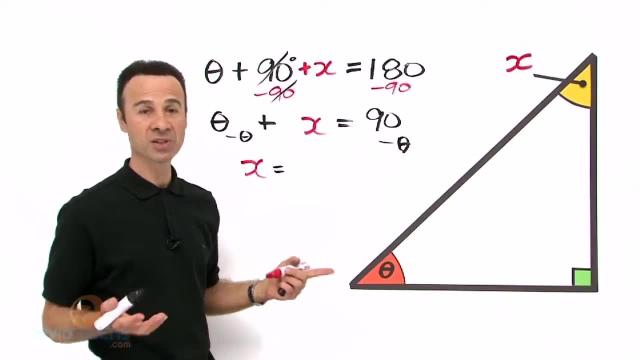 take away theta, alright. X is the subject. now let us see what happens. X equals what do we have here? Well, 90 minus theta. we do not have a number, it is just theta. so let us write that down: 90 minus theta. 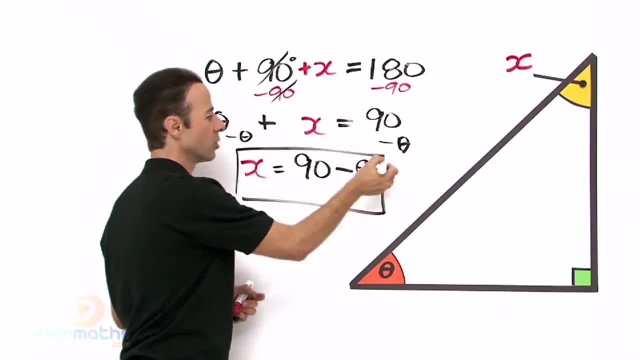 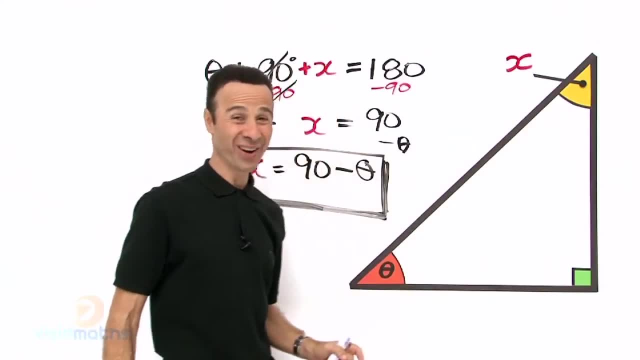 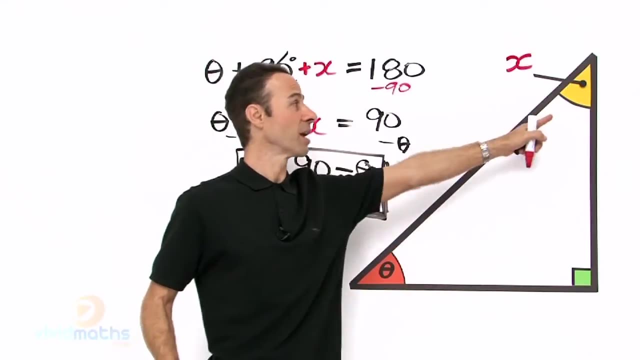 Wow, That is pretty cool when you look at it, because you may or may not have seen this- that pronumeral right up here is always 90 minus that. So no matter what angle you get in here, you just subtract 90 from it and you will get. 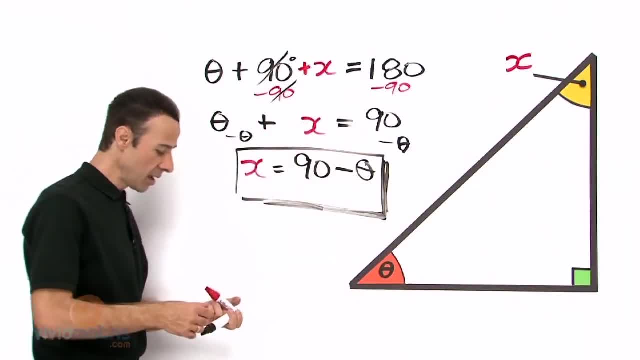 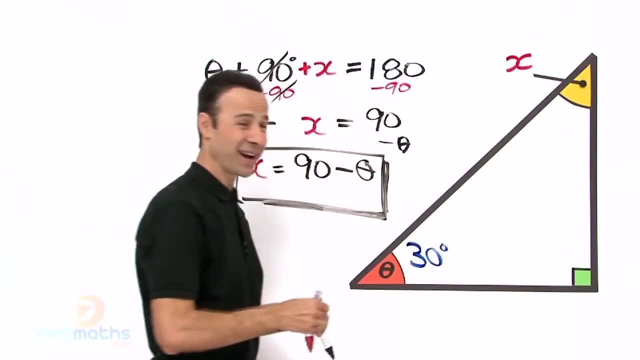 that angle up there. For example, let us say the angle down here was 30 degrees. yeah, Let us make a number up: 30 degrees. and they say: find X up there. what is X? Now that you know what is X, 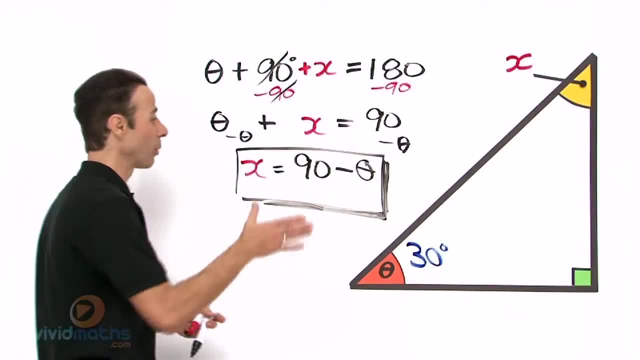 Now, what is 30?? Well, we know the angle sum of triangles is 180 and we know this formula. so all we do to find what X is is simply use this formula. So X, up there for this example, equals X, equals 90 minus 30, which is theta. see that.